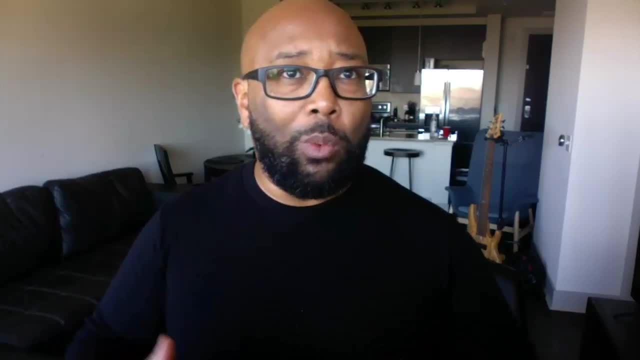 But as a part of that, and what makes a SOC team work and what makes incident response and threat hunting and all that works, is having a good SIEM solution. I'm going to show you how, using a SIEM. one of my favorites Exabeam how this ties together And 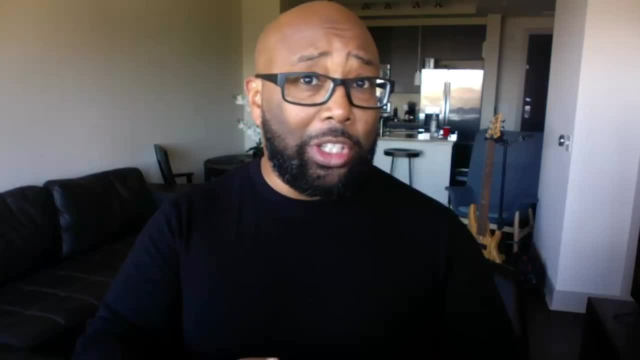 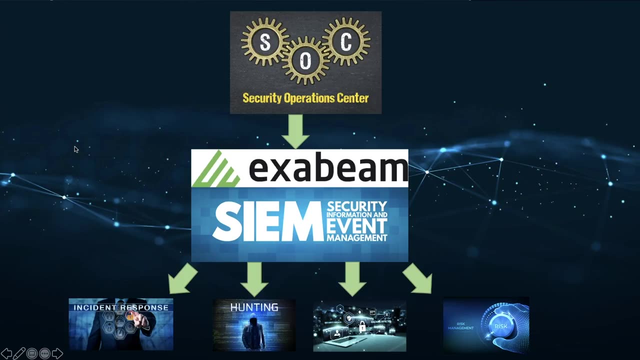 we'll go from the very beginning of where someone in the SOC saw, through the SIEM, a problem, and then we'll look at what the hunting and the incident response would look like. Let's jump right into it Now. what we said is the fact that what you normally see is the SOC is who's responsible? 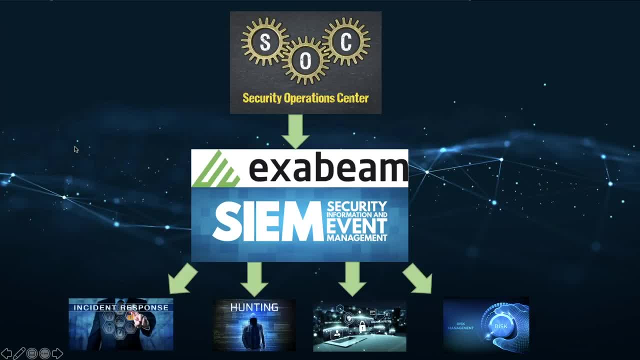 for letting us know where to look for a specific piece of malware. So what you see here is kind of my way to illustrate this. You can see the SOC up here at the top. These are the unsung heroes, the people that are in there daily grinding it out, looking for these variations and anomalies. 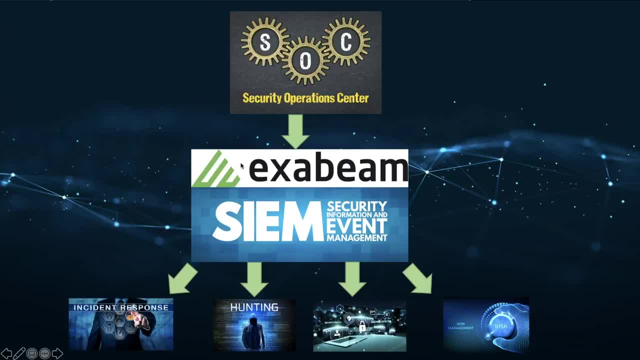 And then they're usually plugged into what we call a SIEM or a security information and event management system, And one of my favorites, as I said in the previous part of this video, is Exabeam. Now what you can see is incident response, threat hunting. you know, incident response and threat hunting. 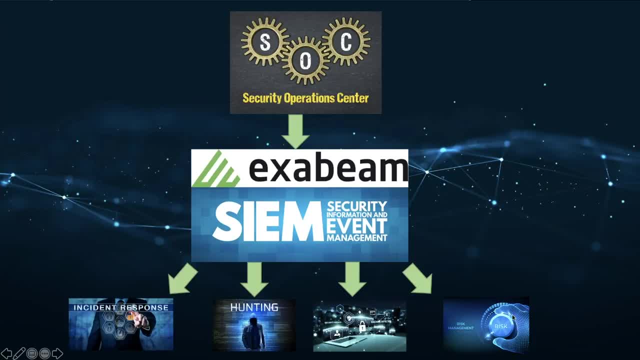 Incident detection or intrusion detection, risk management. all of this ties into these SIEM solutions and utilizes the data. Let's look at what happens in a scenario- And we're going to go quickly from beginning to end- to where something in the SIEM showed us that something wasn't quite right. 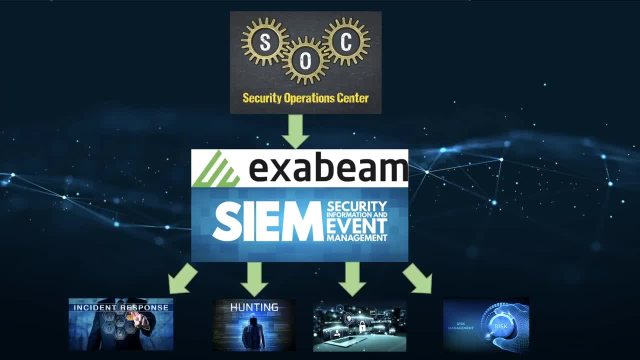 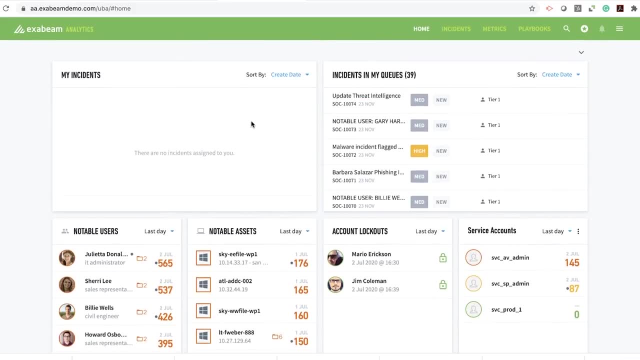 And then we'll dig into the weeds so you can see how we get into those weeds- Kind of counter to what my normal videos are, whereas we pick up right in the weeds. Let's look at that. So I've logged into my Exabeam. 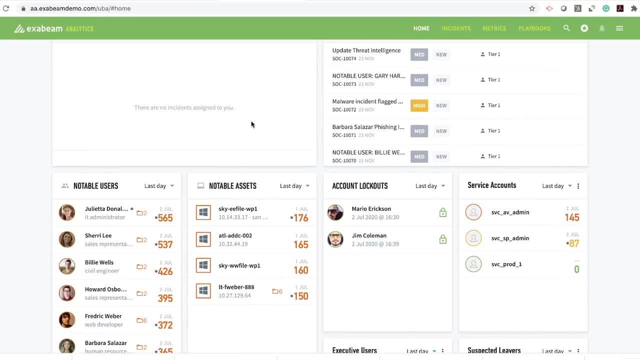 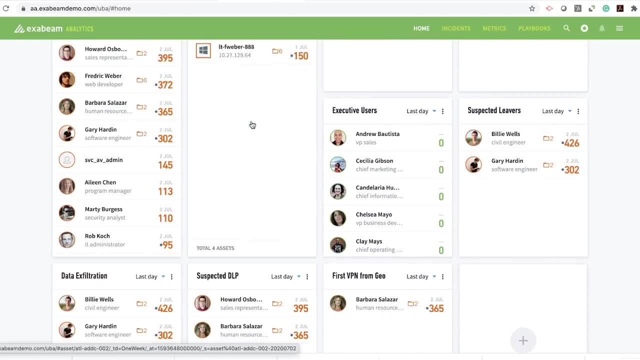 Exabeam SIEM console here And you know this is one of the best dashboards, most intuitive dashboards of the SIEM market. You know this is one of my favorites. So, as you can see, here we can see all kinds of things. 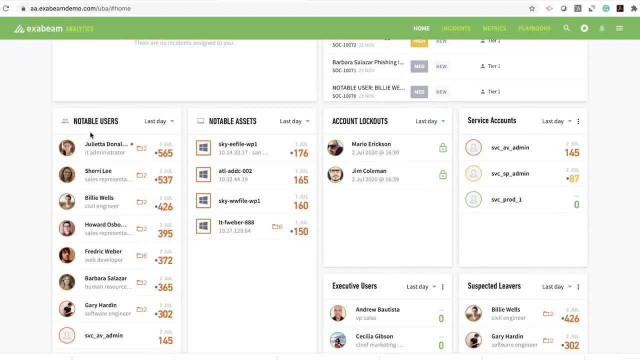 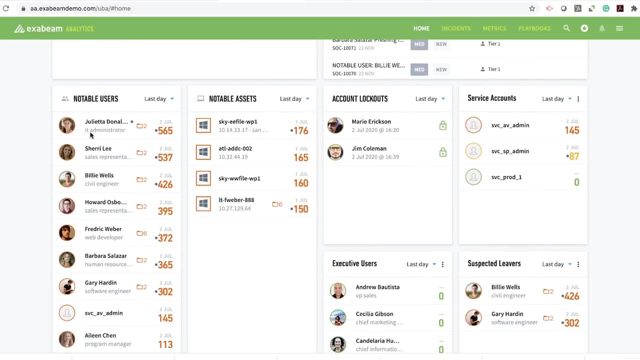 We can see notable users- And by notable we mean users that there's been some activity that makes us notice them. You know, there's something about this user's activity that makes us kind of put them in this category. There's notable assets. 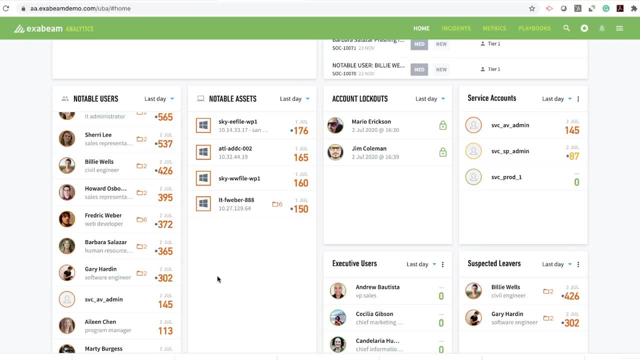 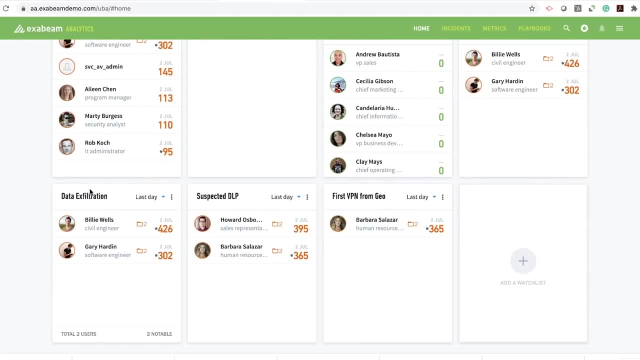 This would be specific servers or desktops or things like that That may be doing some behavior. that kind of makes us notice those devices as well, And you can see we have all different kinds of categories here that we look at in our SIEM to see what's going on. 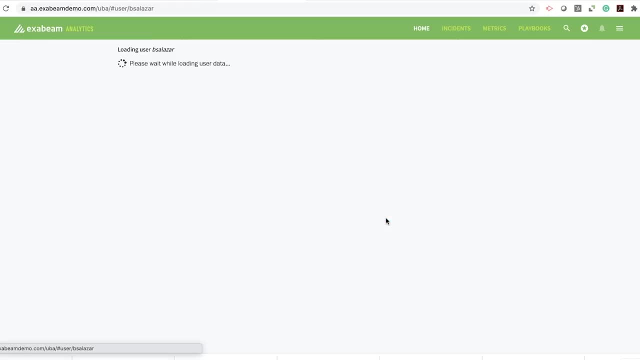 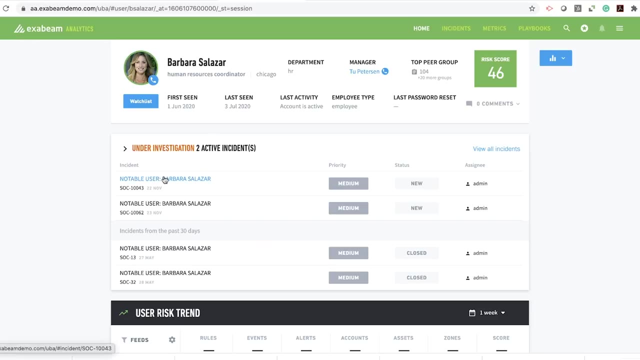 Now, in this particular instance, we're going to look at Barbara Salazar here. So if we go look at her alert and see why she's in the notable people's list here, we can see if we click on this incident here. 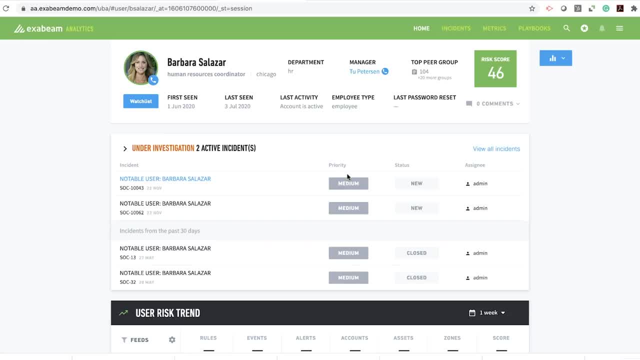 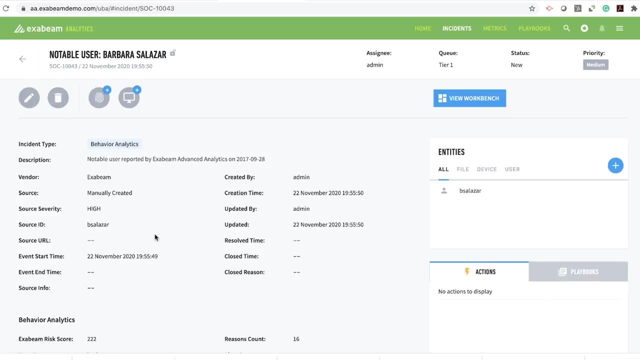 Now I want you to notice, this is classified as a medium. It's not a critical, not a high, It's not a categorization. But if we go look at her and look at what this report is, what we see- and this is November 22nd- 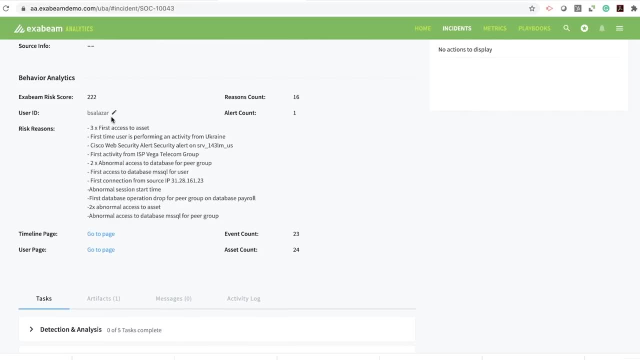 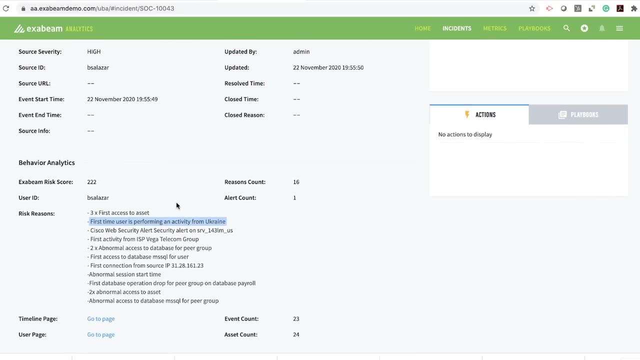 So this is like just you know, yesterday What we can see is Ms Salazar here has been VPNing in from the Ukraine, And the reason she got into this group of notable is because she's never VPNed from the Ukraine before. 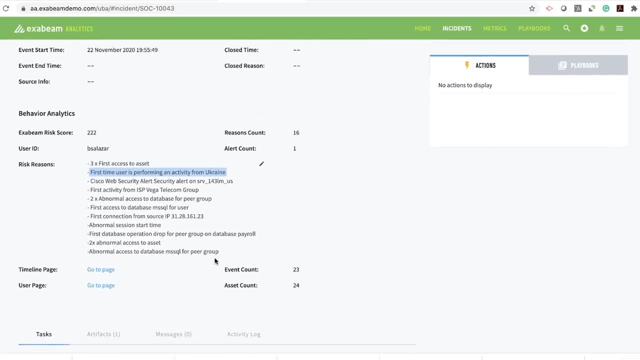 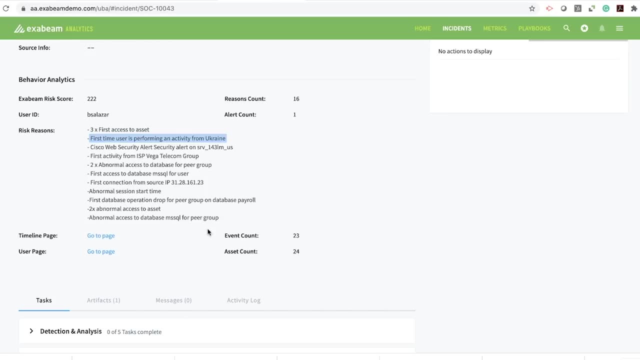 Right. So that may not be anything, but it could be everything. So that's how we got to focus. So now we're going to go and look at our VPN concentrator or our VPN drop box or jump box. So you know, a lot of these organizations have these really old boxes or really old infrastructures where when you VPN in, you jump off into that box. 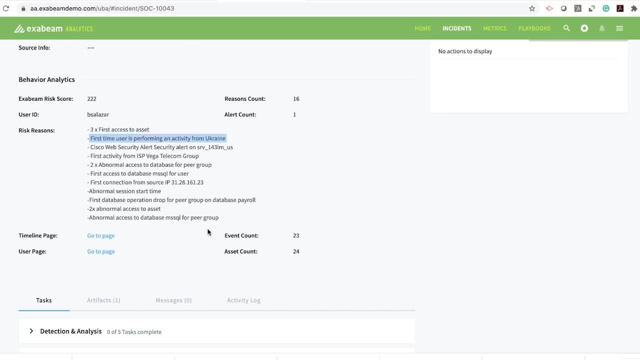 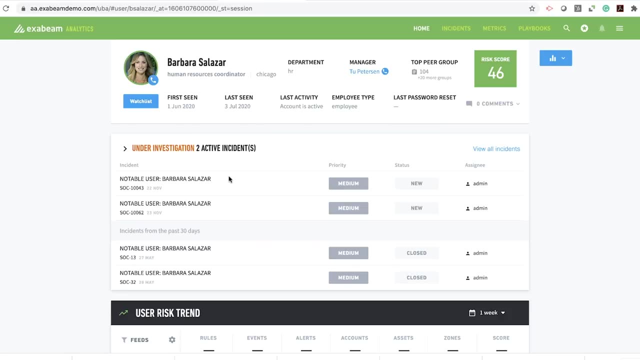 And then from that box, you can move horizontally inside the environment. So now let's jump over to that, based on what we saw in this great dashboard here to get us to that point to where we knew that Barbara Salazar was having an issue. 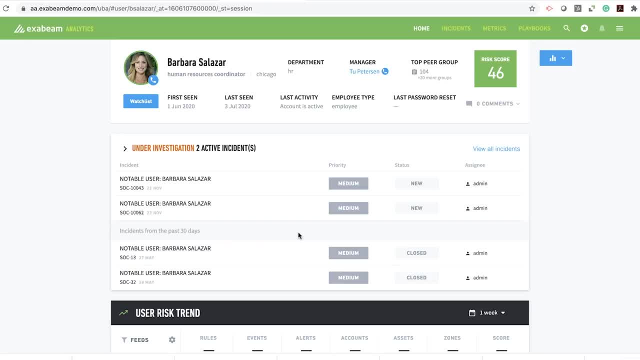 Or there could have been an issue And this could be the impetus for where we might start something like a cyber threat hunt based on just this medium thing. here We don't know that there's anything wrong, but the dashboard can quickly get us to the point. 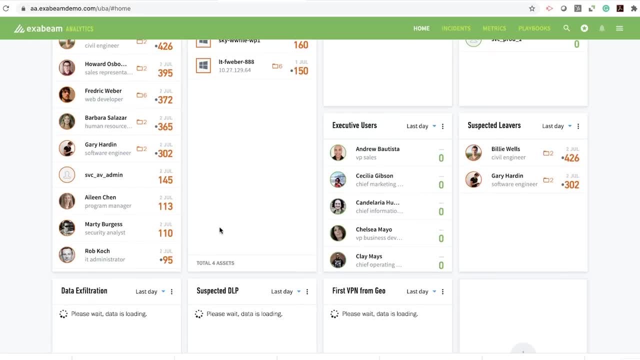 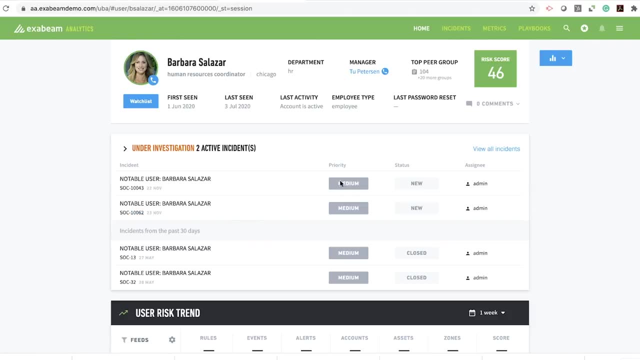 Remember we started here. It can quickly get us to the point to where we can kind of see that, okay, there's VPN from a geolocation that she's never done before. We don't have any evidence of malware or anything like that. 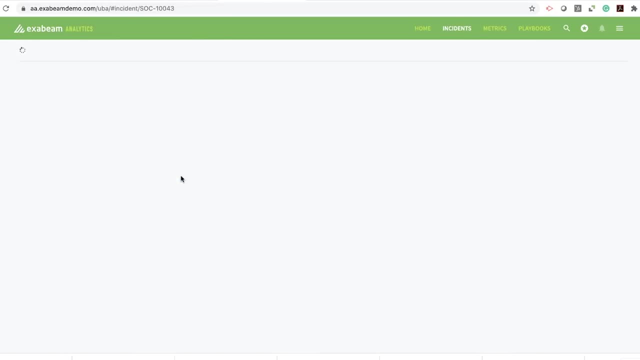 It's a medium priority thing. But you know what? Let's create a threat hunting hypothesis And assume that maybe there is an issue because there's a VPN from the Ukraine. This gives us all that. So let's go now and look and see what we would see on her VPN session or the previous sessions that she's generated. 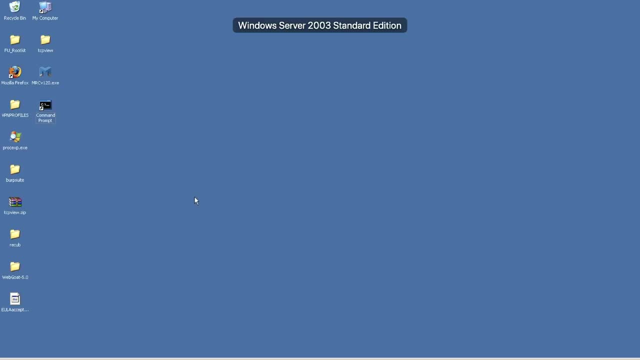 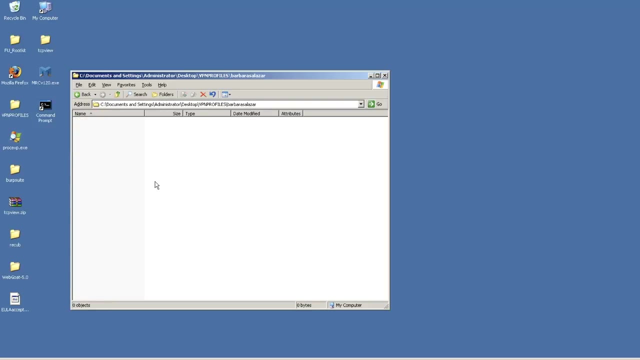 So now, as we get to the VPN junction point, you can see the VPN profiles here And if we go look at those, we look in her profile and we don't see anything weird there. But we're forming an hypothesis here And because we understand that the whole purpose is to create a threat hunting hypothesis, 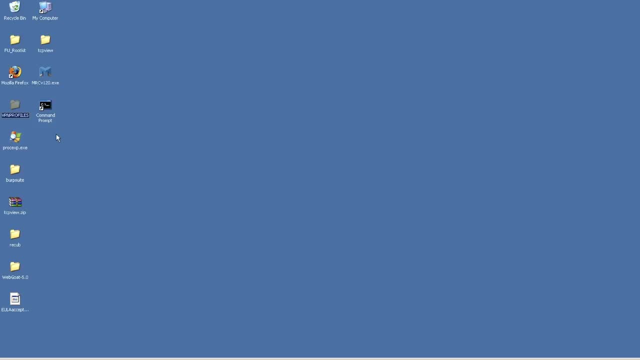 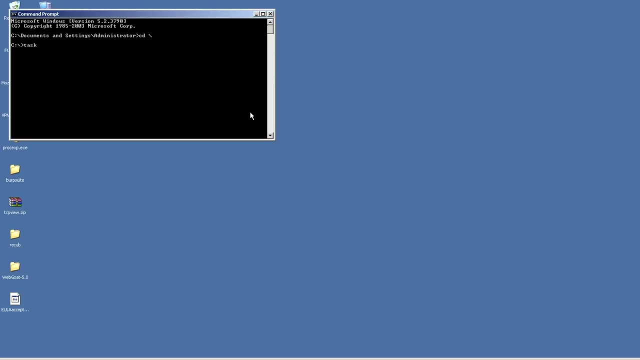 And even if we don't have any evidence of any of these advanced persistent threats is they don't want you to see evidence of anything going on. So just out of curiosity, here We're just going to run, I'm going to run a task list and get a list of running processes. 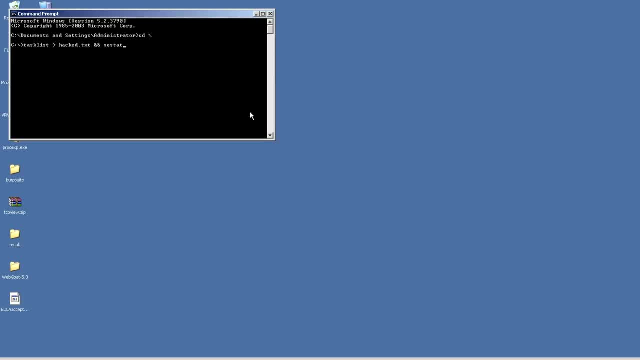 And I'm also going to run. These are just built in one of these commands. I'm going to do net stat current connections And I'm going to write that to the same file. All right, Now this is a common little triage that I'll do when I think something's wrong, And I'm going to copy this file somewhere. 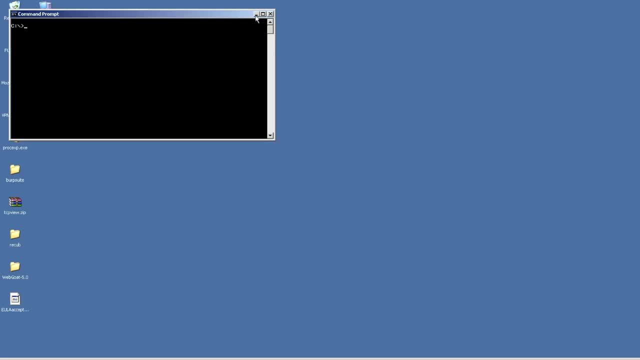 that I can get to it remotely, All right. So we don't know that anything's wrong. but we just did a little triage. We copied that file over, took a list of you know what was running and just to show you what that file looks like. It's just a little file looks like. that shows us running. 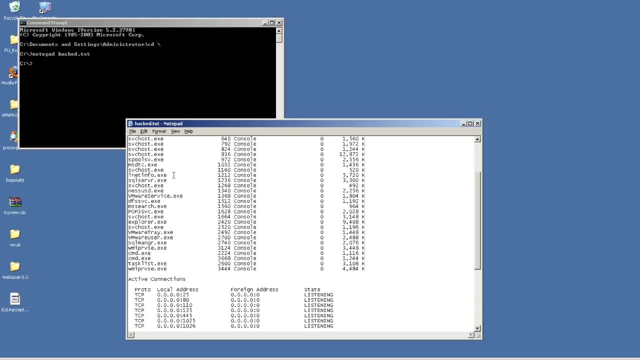 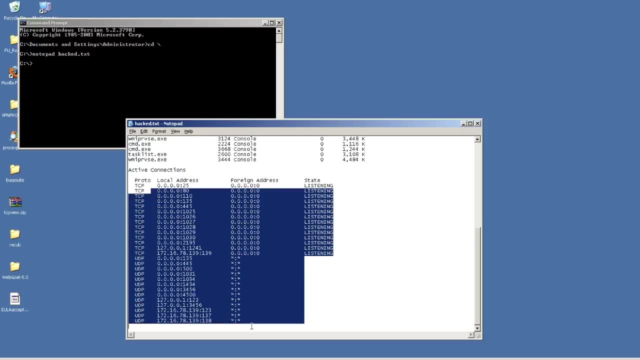 processes and connections. Now notice, here's a list of all the running processes and they're all legitimate. One of this process is: nothing looks out of whack there. Here's, you know, connections. There's no weird connections, There's actually no connections, just listening ports. 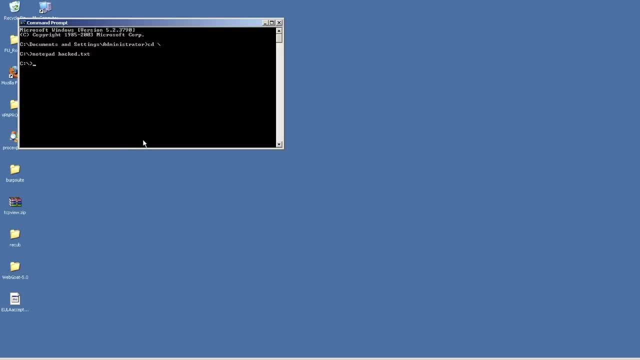 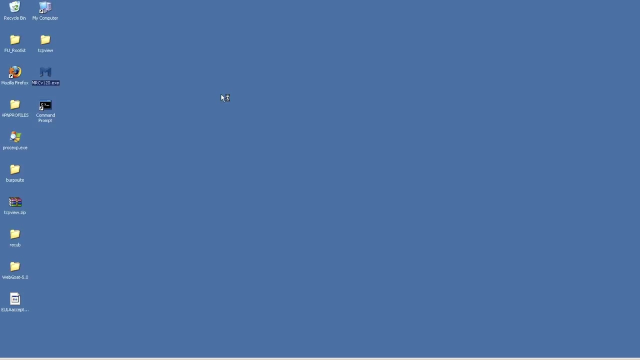 They all look legit. So nothing to see there on this jump box. Now, because we saw, got that hint from Barbara Salazar's VPN from the Ukraine. we knew it came into this box. We're going to just as a precautionary measure, out of an abundance of caution, we're going to take a memory dump anyway. 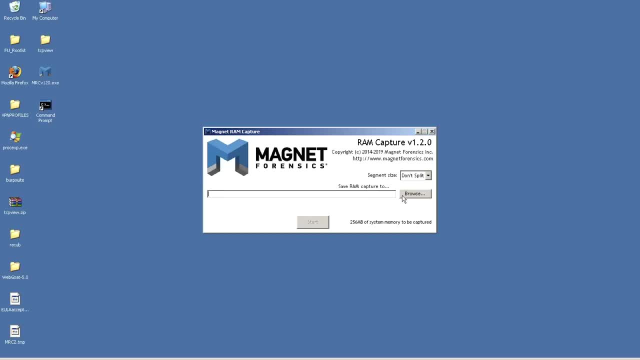 of this machine And we always talk about the order of volatility and why that's such an important thing. So we're going to write this right right onto the C drive here And we're just going to write a memory dump out- And I'm using this old machine because it's got a really 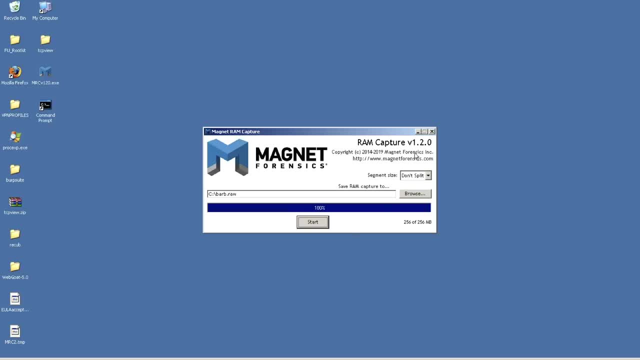 really tiny amount of memory. So this, this demo can go quicker, with me just taking like a 256 meg memory dump. But you get the point. You don't have to sit here and watch me. you know, wait for a memory dump from a 32 gig memory. 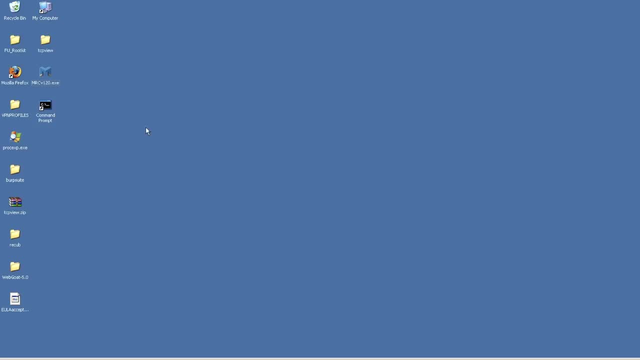 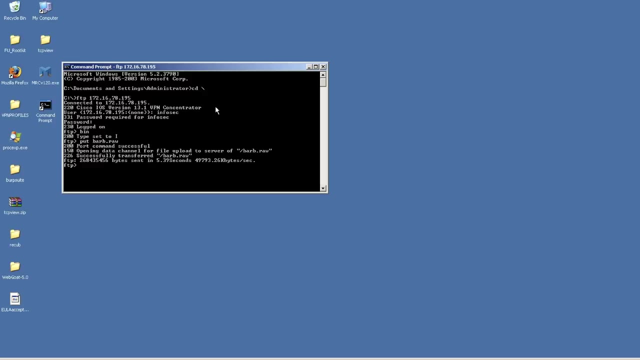 machine to take 45 minutes for you to get the point of what's going on here. So I'm going to take that memory dump now and we're going to put it onto a server. All right, it's transferred. So now we're going to go to our investigative machine, we're going to bring that memory dump over And 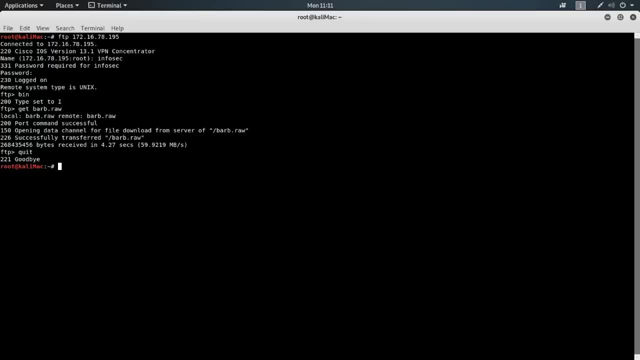 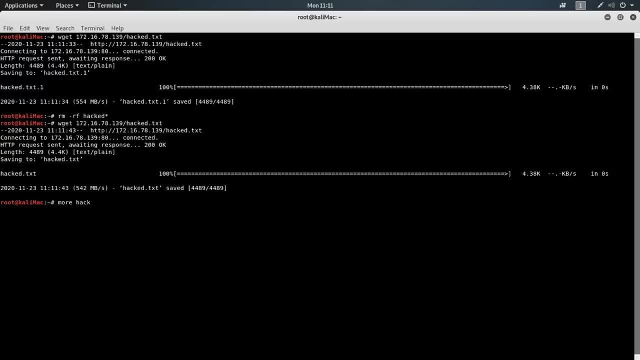 then with that dump, we're going to just do a comparative analysis here. So, remember, we wrote out this file And then we're going to take that memory dump and we're going to put it onto a server. So we wrote out this hacked file, right, that showed us everything that's going on on the. 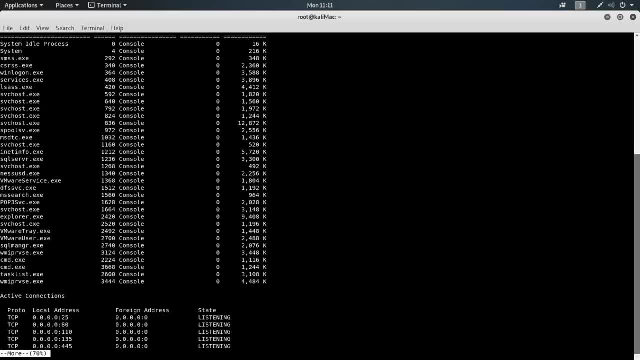 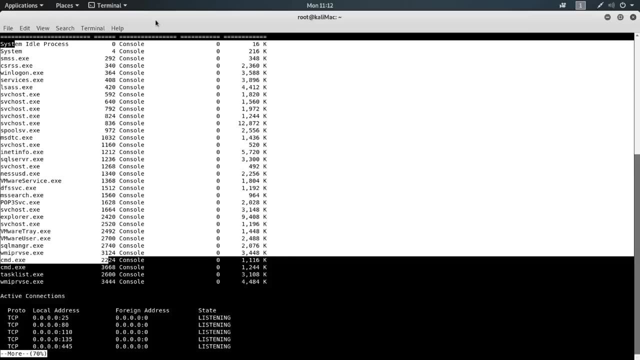 machine And we can see. there's our running processes And then we can see run under our connections. I want you to pay attention to the fact that there's a listening session on port 80 and port 110, but nothing on port 100. And here's again the running processes. Now, taking that, 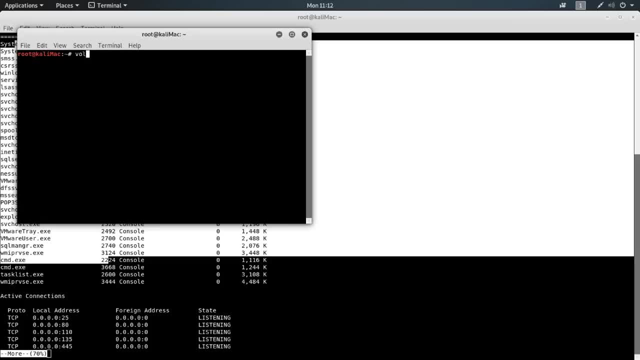 memory dump that we just bought over. So let's look at that. I'm going to use a tool called volatility, So memory dump tool, And we're going to point at that barbraw file here, All right, and just not trying to teach you volatility here. So I'm not going to go into all the things that I'm doing. 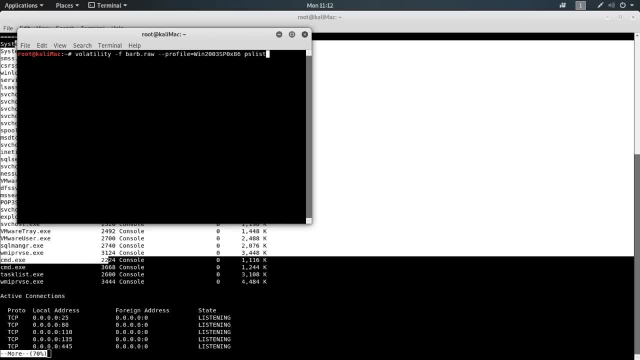 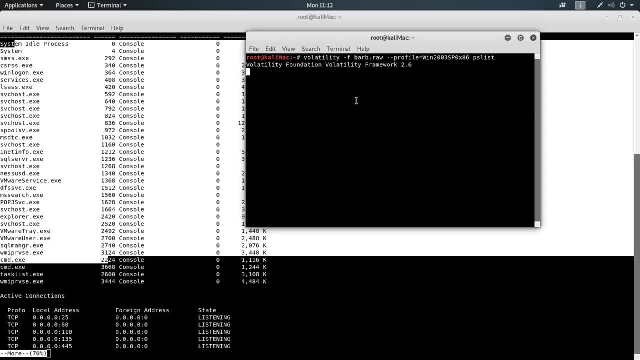 with the commands here And we're going to get a list of running processes. So that's going to be the first comparative analysis we're going to do. So we're going to look at the processes that are currently running per the memory dump and compare that to what we see when we run task list or task. 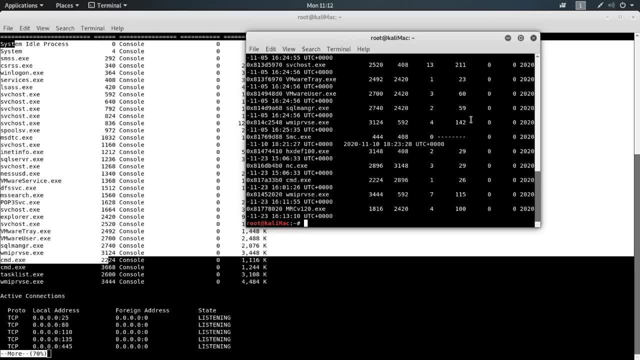 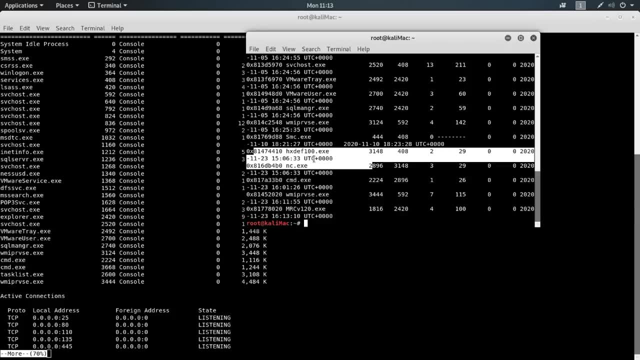 manager from the victim itself, which is what we see over here And right away we see two processes right there that we don't see running on the other side of here. So the machine itself is lying to us and telling us that you know, this is all the processes. 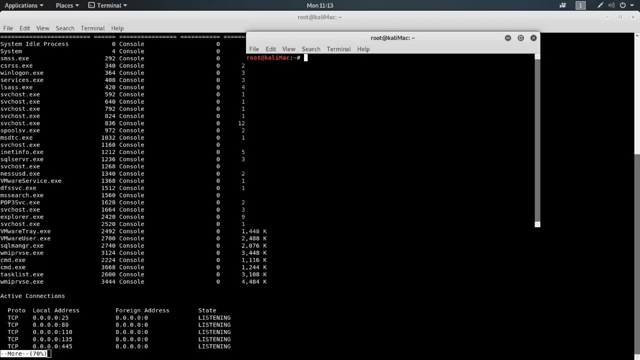 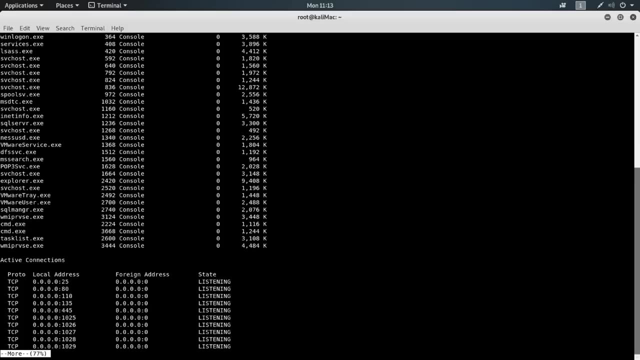 we have and there is no weird connections. But also, if we look at connections we'll see that there's a connection on port 100 that doesn't show up over here. right When we looked at the listening ports from the machine itself it says: look, we don't have any. 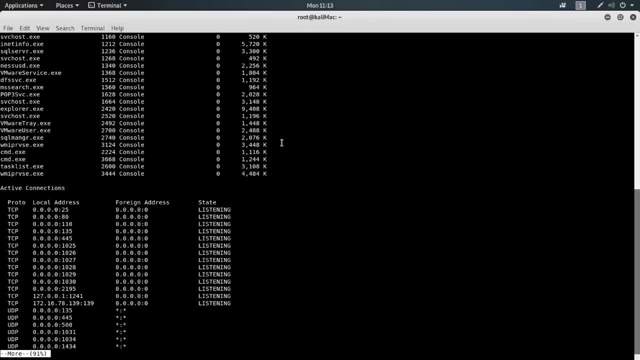 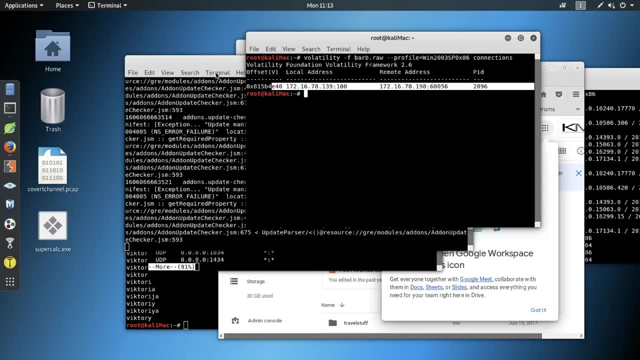 connections And this is what's all. it's listening, So clearly there's something wrong. You know what it ends up being is. that weird process is actually a rootkit that you saw there. So that's actually a rootkit that's running, And if we extract that rootkit, we would find that. 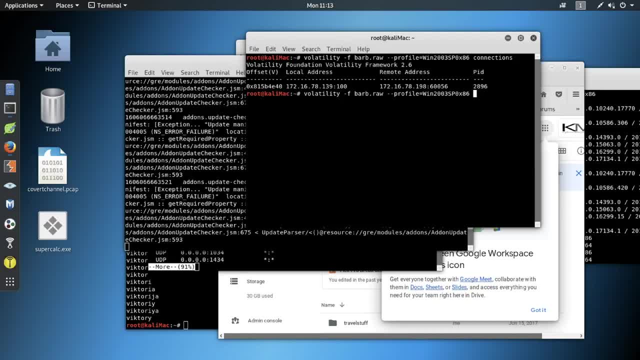 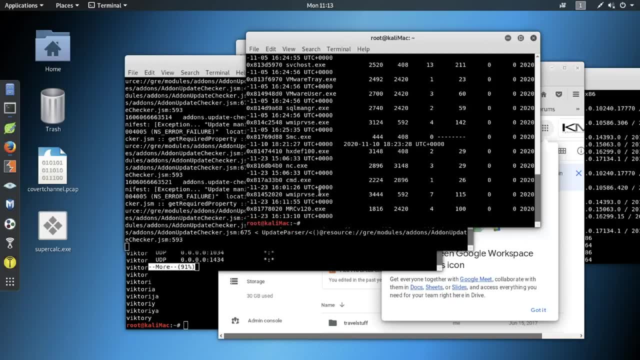 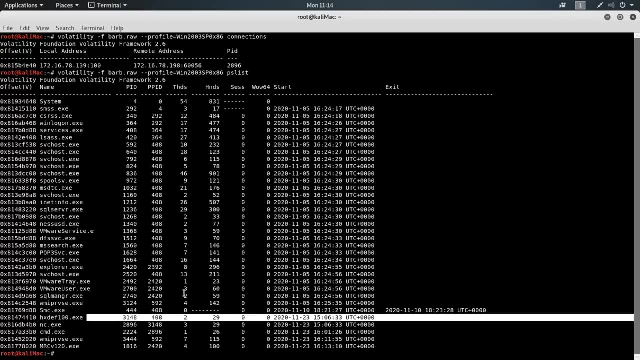 it's something very, very bad. As a matter of fact, let's go ahead and do that. So let's get the process name for that rootkit And it's and it's PID. All right, so that rootkit, That thing that we think is a rootkit which is right here- All right, that's running as a PID of. 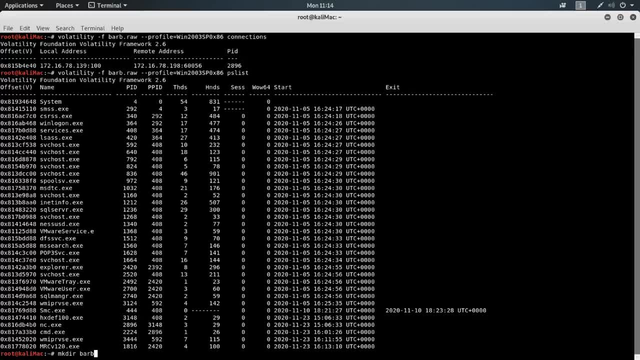 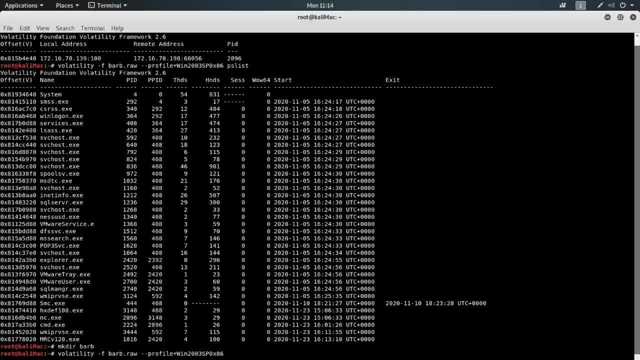 3148.. So what I'm going to do is make a directory named barb And I'm going to extract that rootkit out to that directory And we'll use something called proc dump to do that. from volatility We're going to dump it right to. 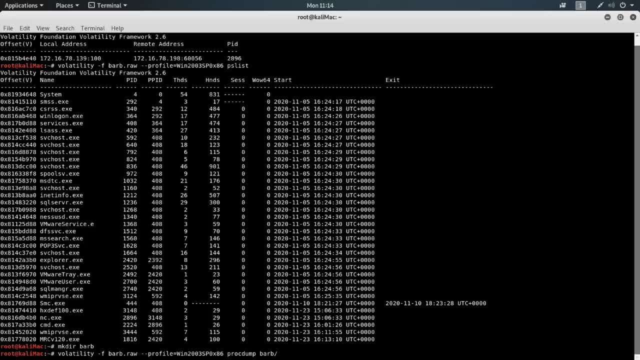 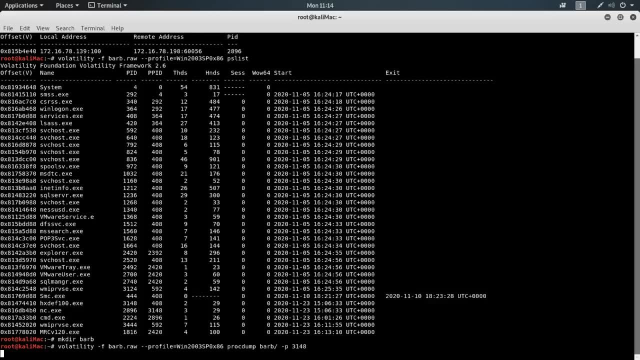 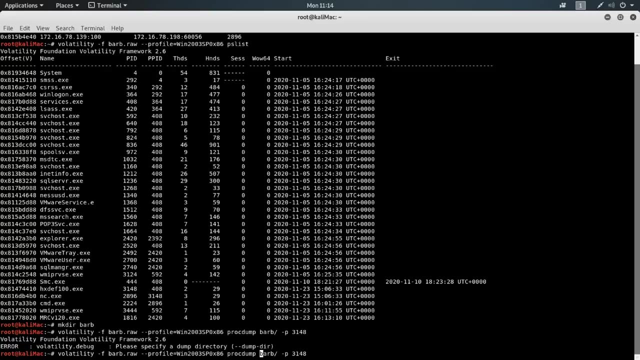 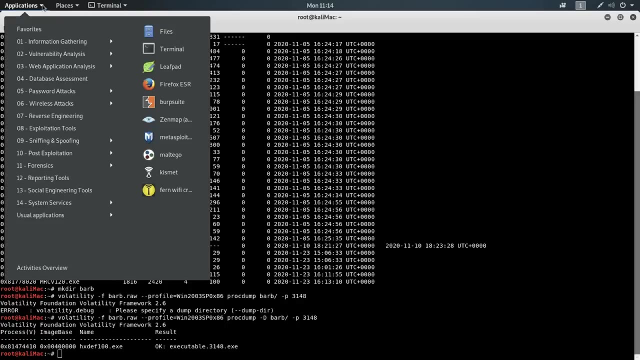 barb, And that process is 3148.. Oh, we forgot to do our dash D here, my bad, All right, so it dumped it out. I'm just going to go right out to now. Now, in practice, we don't. 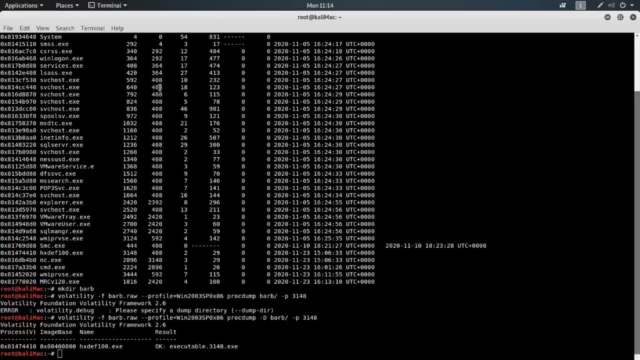 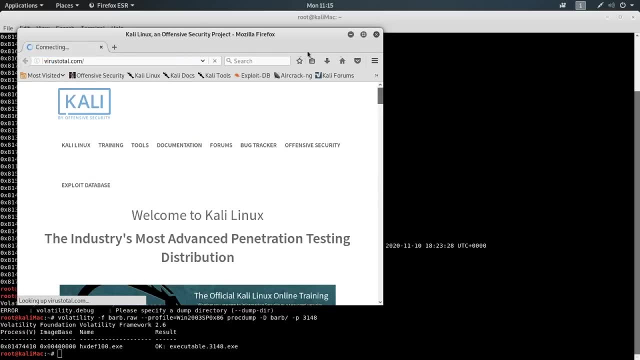 use virus total for real work, Because you know there could in this rootkit there could be, you know, customer information exposed or something like that. So but just for this demo I'm going to show you that that rootkit is really bad. 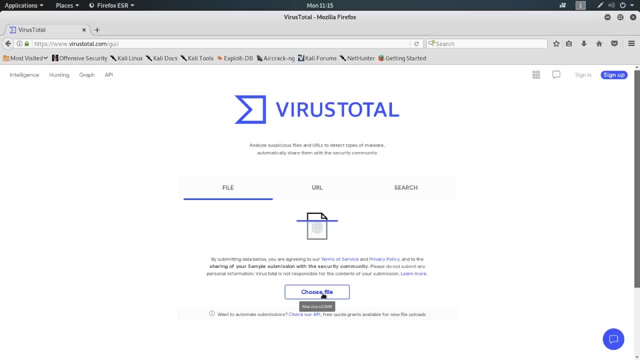 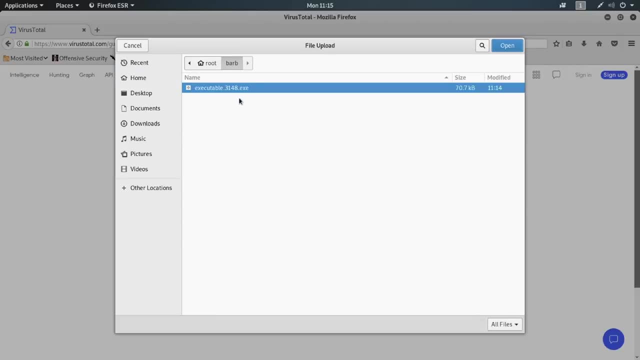 it is something bad And it doesn't show up on any scans or anything like that that you do. So we had to actually do the memory dump to get to this. And then there's the binary, So we go ahead and upload it to virus total and let virus total tell us what it thinks. And, of course, 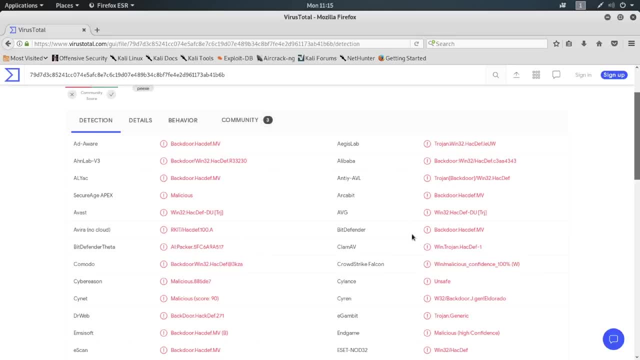 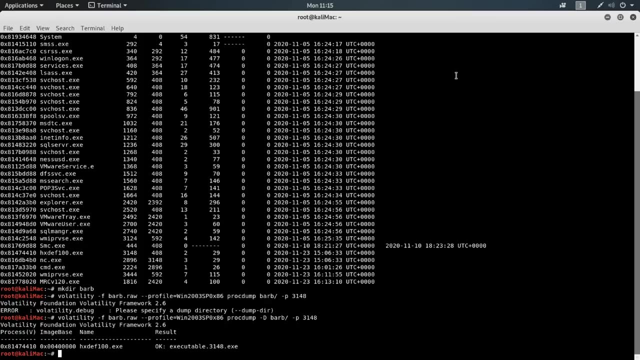 it comes back and says backdoor, backdoor, rootkit, rootkit, rootkit, bad, bad, bad. The point of this is, generally we start in the weeds here, But we knew to do a memory dump. we knew to look for disparities or differences based on what the memory said versus what the 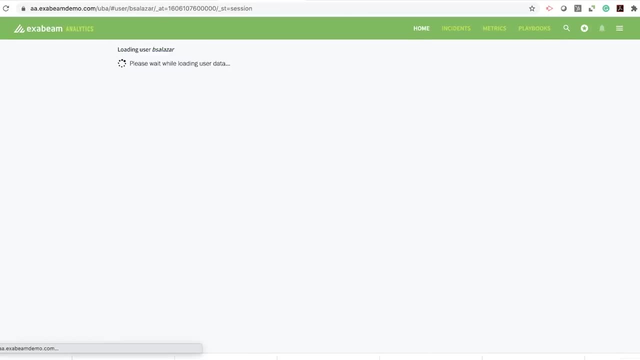 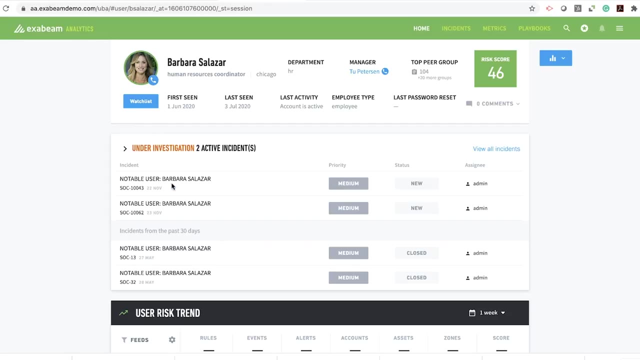 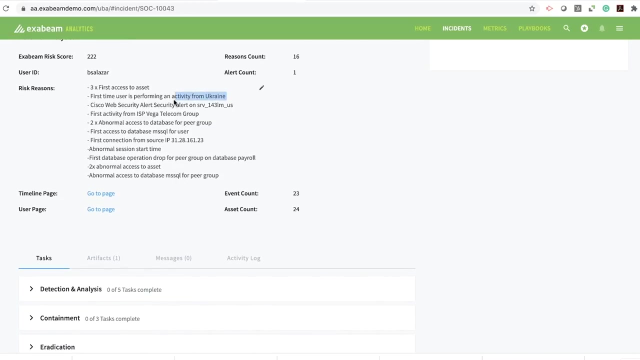 machine said itself. All because in the beginning, when we looked at our sim, we knew that something was up with Barbara Lazar's VPN sessions, because why She was doing VPN sessions from somewhere she'd never done them before, In this case, the Ukraine- And that